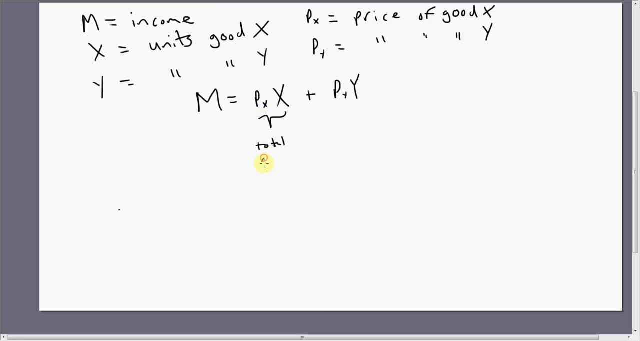 This right here is just total spending on X. Total spending on good X. This right here is total spending on good Y. Price times the quantity purchased. Total spending on good X And Y. When we do our budget constraint graphically, we'll put the Y good up here. 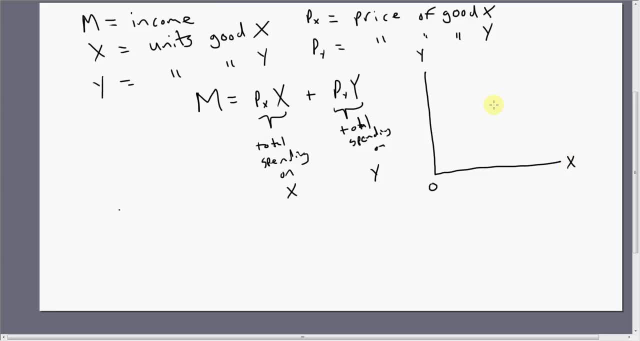 The X good. down here These are. again, we're measuring units here. These are physical units. Good X, physical units of good Y. So to get an equation that describes a budget constraint, we want to solve this for Y, So I'll go over here and solve that for Y. 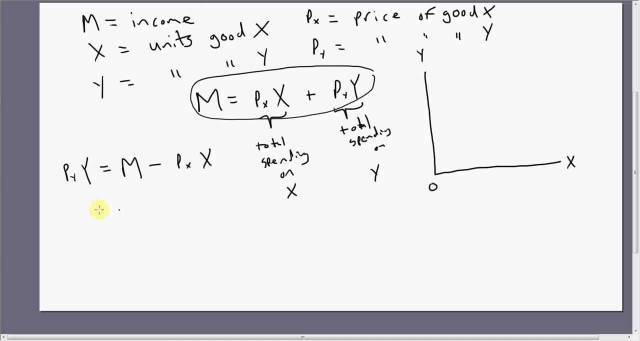 So just moving this price times X term over to the other side, I'm getting rid of the price of good Y here on the left-hand side by dividing everything through by the price of good Y And we're left with an expression for the budget constraint. 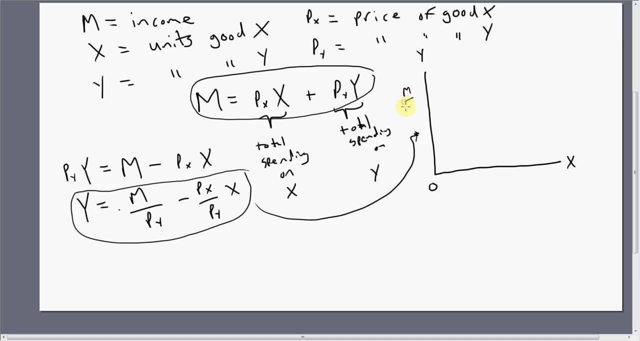 The vertical intercept is right here. Just take your money income and divide it by the price of good Y. That will be the maximum number of units of good Y that you can buy. This is going to be a downward sloping line. Notice the slope here is negative. 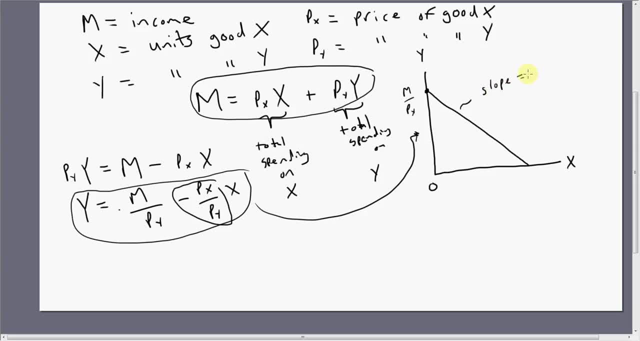 And the slope just reflects the ratio of the two prices minus the ratio of the two prices. So the price of good X divided by the price of good Y is going to represent the slope here, And the other thing that we can get here is a horizontal intercept. 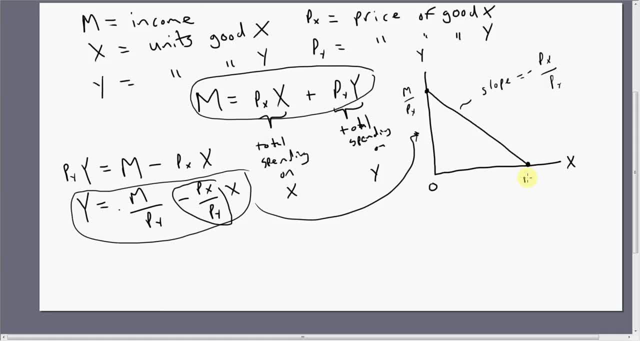 The horizontal intercept is just going to be M divided by the price of good X. You can figure that out by just setting Y equal to 0 here or here, Setting Y equal to 0 and solving for X. That's what you'll get. 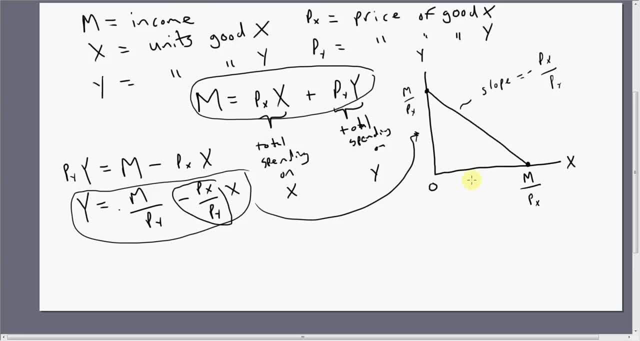 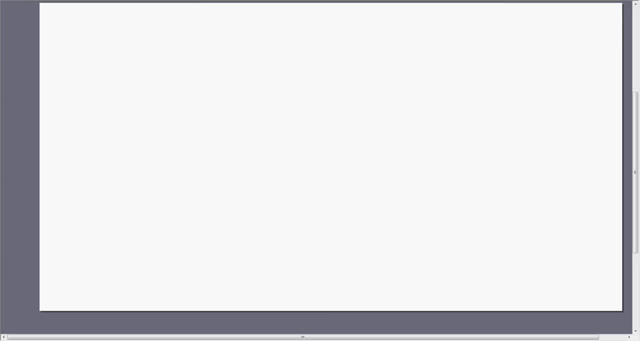 So that is the basic idea of the budget constraint. Now let's do some examples with numbers. Maybe the consumer has $100 of income. The price of good X is $2 apiece. The price of good Y is $4 apiece. 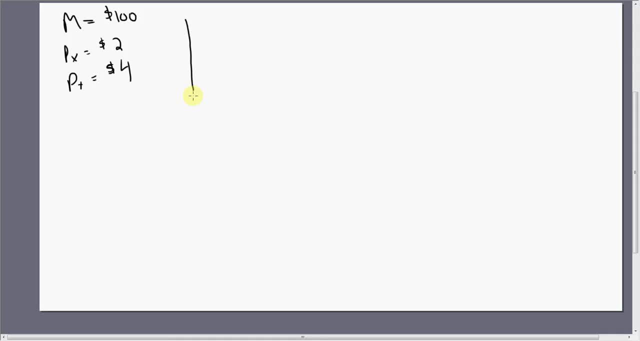 Let's graph the consumer's budget constraint. Let's graph the consumer's budget constraint. So what we learned from the previous slide is that the vertical intercept is going to be your money, income divided by the price of good Y. So 100 divided by 4 means at most. 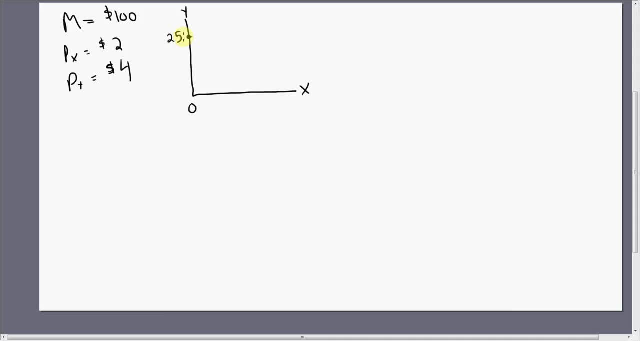 we could get 25 units of good Y. We've got $100, and good Y costs $4 apiece. So at most we could get 25 units of good Y. As for good X, we've got $100.. We've got $100.. 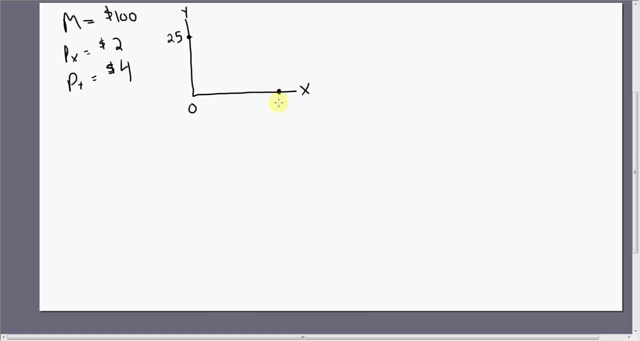 Good X costs $2 apiece. so 100 divided by 2, we could afford 50 units at most. Connecting the dots here we have our linear budget constraint And notice that the slope rise over run. 25 divided by 50,. 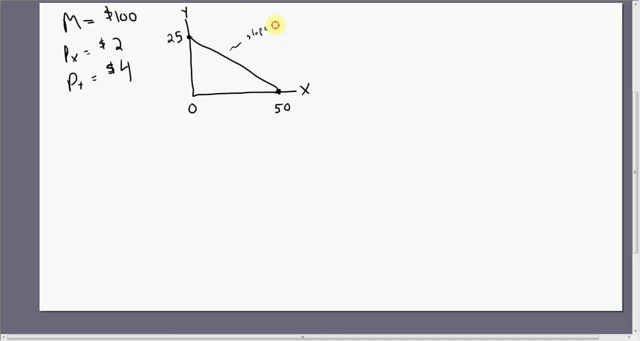 are just a ratio of the price of good X to good Y just minus 1 half. Alright, what would happen if money income doubled, the price of good X doubled and the price of good Y doubled? What would happen to our budget constraint? 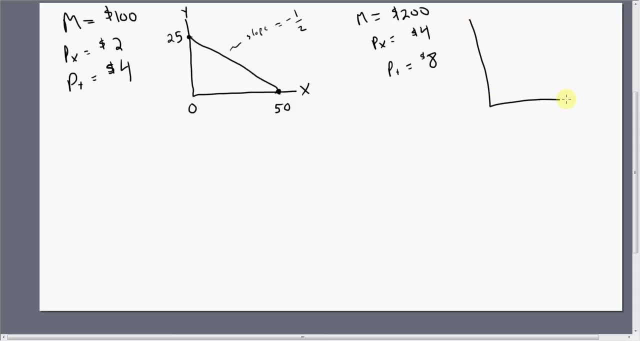 Well, actually nothing would happen. It would look exactly the same. A doubling of income and a doubling of all prices leaves the budget constraint unchanged. Down here, this is going to be 200 divided by 4. We can still only afford to buy 50 units of good X. 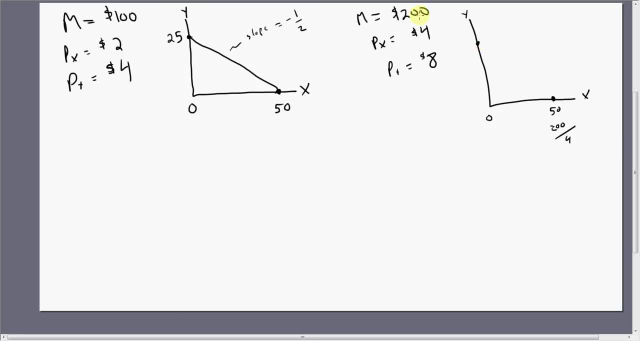 Up here the vertical intercept income divided by the price of good Y, 200 divided by 8.. At most, we can still afford only to buy 25 units of good Y. So these two budget constraints are exactly the same. Okay, let's do something, maybe a little bit more interesting. 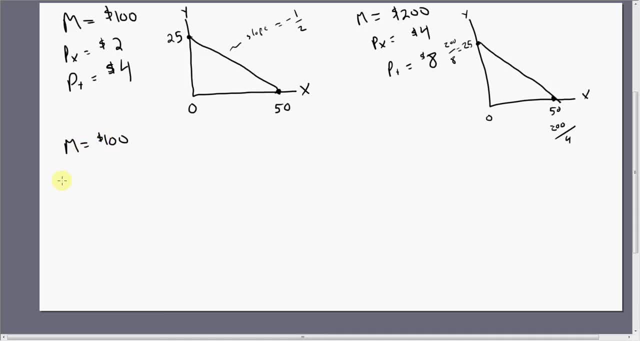 Going back to $100 of income. price of good X rises now to $5.. Price of good Y is unchanged at $4.. Let's see how this budget constraint changes from our original. We still can only afford to buy 25 units of good Y. 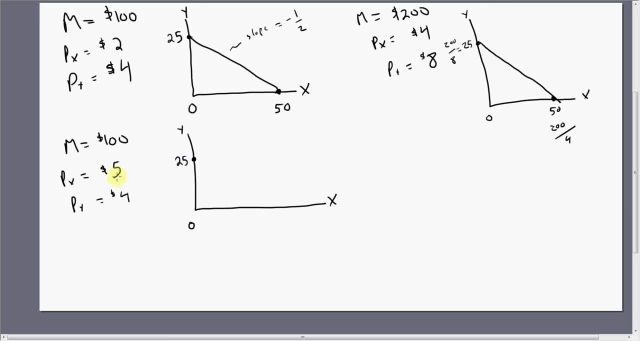 at most. But since good X increased in price from $2 to $5, we can now only afford to buy 20 units of good X if we spent all our budget on good X. So 100 divided by 5 means at most we could get 20 units of X. 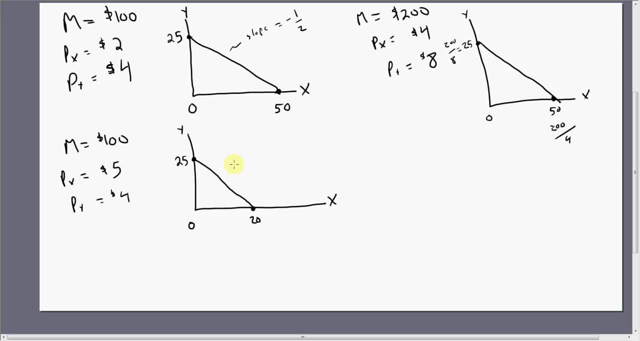 if we spent all our money on that good. So this is what our budget constraint would look like in this case. Notice when the price of good X increases, this budget line it pivoted in. It went from 25 to 50 here to. 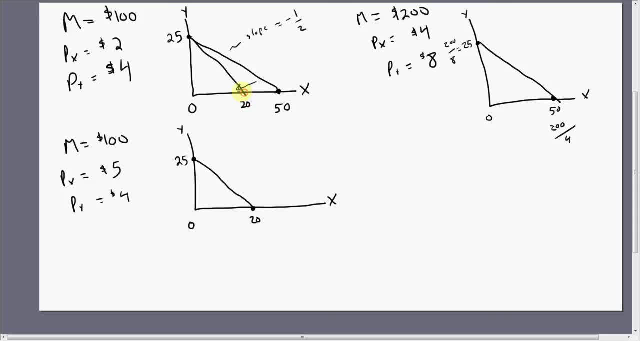 oops, not quite drawn to scale, but 25 to 20.. Alright, let's look at another example. Let's say that M equals $100, and the price of good X is our original $2 a piece, but now the price of good Y is lower. 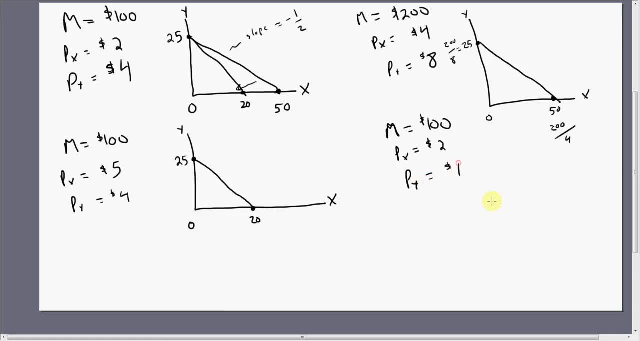 The price of good Y fell to $1.. In this case our budget constraint will be 100 at the vertical intercept, 100 divided by 1, and the horizontal intercept is unchanged. So when the price of good Y falls, notice that the vertical intercept, it increases. 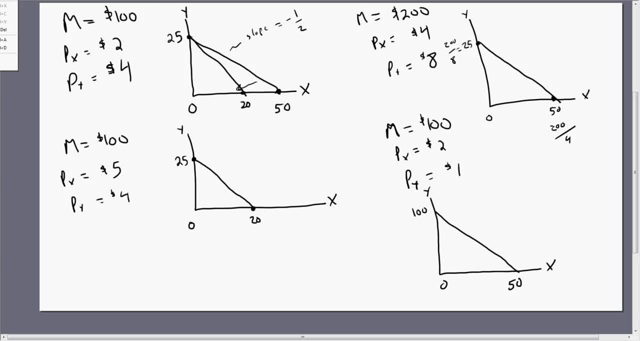 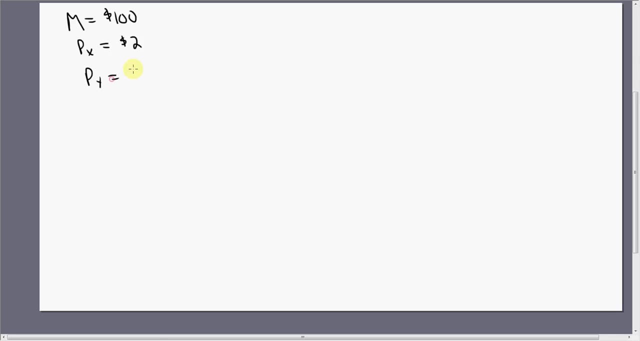 Alright, let's do a few other, maybe more interesting examples. Okay, so let's start with this, This setup. but now let's assume that we have a buy one, get one free offer for good X. So with good X, there's a buy one, get one free offer. 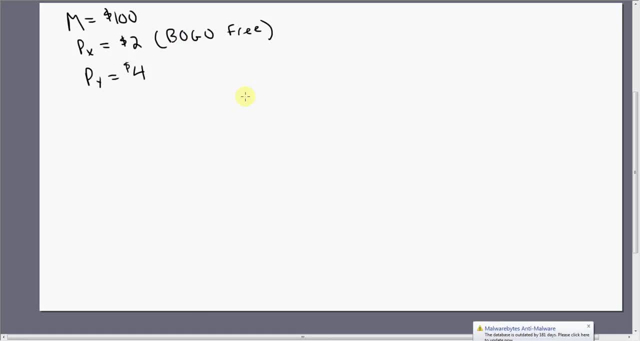 So, BOGO, buy one, get one free. What would the budget line look like in that case? budget constraint: Well, if we spent all our money on good Y, we still could afford only to buy 100 divided by 4, or 25 units. 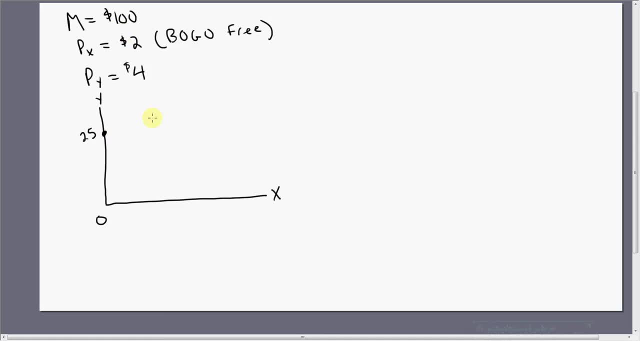 Okay, income divided by the price of good Y gives us this point: If we spent all our money on good X, we would buy 50 units, but then we'd also get 50 free, since it's buy one, get one free. 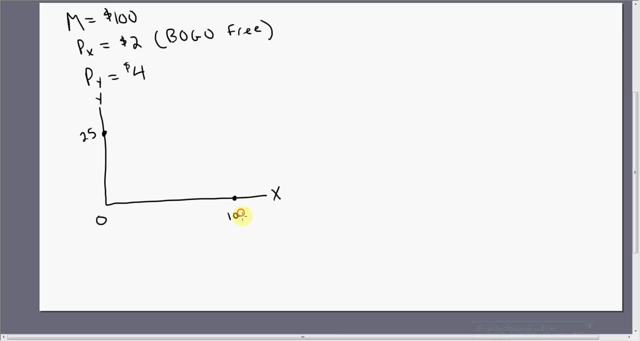 So we could now get 100 units of good X in total. You can afford to buy 50 for $2 a piece, given you're $100, but since it's buy one, get one free. you get 50 free and your budget line will look like that. 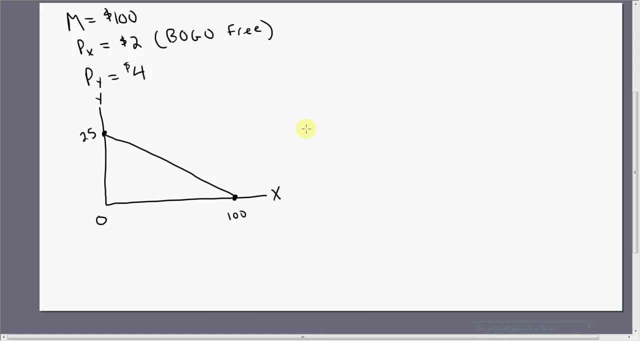 or your budget constraint will look like this: Okay, let's do some other examples that you might encounter. You got an income of $100, price of good X is $2, price of good Y? price of good Y is $4. 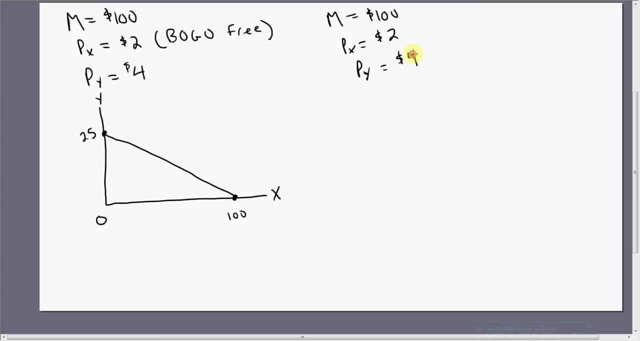 But now, let's say you have a coupon that gives you 10 free units of good X. You have a coupon or voucher that gives you 10 free units of good X. Let's think how that's going to work in this case. So if you spent all your money on good Y, 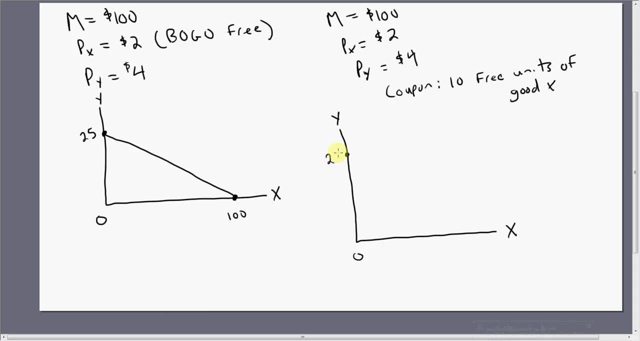 $100 divided by 4, you could buy 25 units of good Y. Then you could use your coupon to get 10 free units of good X, which is going to be a point right here. So this consumer could be at a point like this. 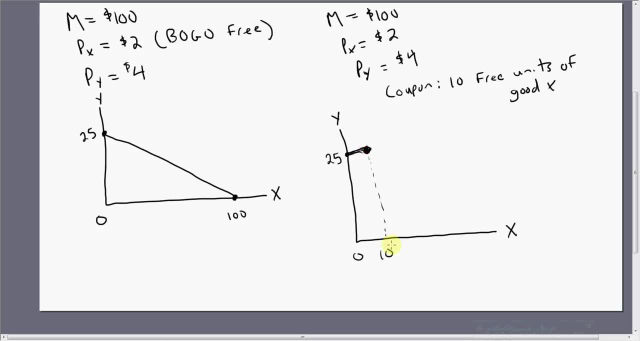 consuming 25 units of good Y and 10 units of X. So if you spent all your money on good Y being able to buy 25, use your coupon to get 10 free units of good X. Okay, so we get this point. 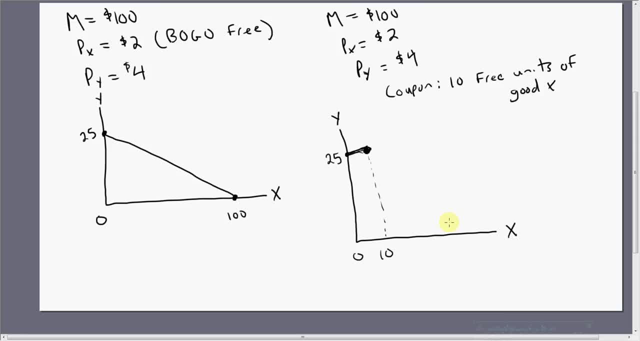 Now let's think about it from the perspective that the consumer spends all his money on good X. If you spend all your money on good X, you could buy 50 units of good X. use your coupon 50 plus 10, that means you'll be able to consume 60 units of good X. 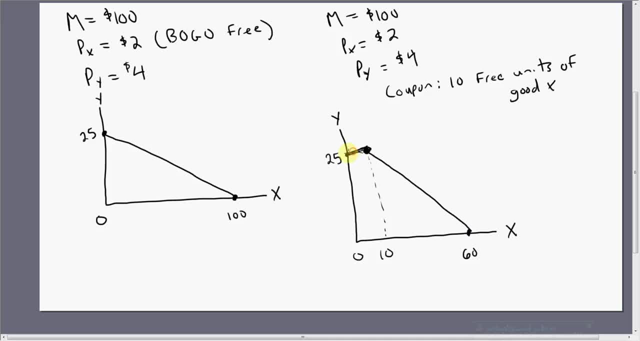 So this is what the budget constraint looks like. in this case There's a kink in it because of this coupon. okay, Let's do another example. get another kink in the budget constraint: M equals $100 as before. price of good X equals $2,. 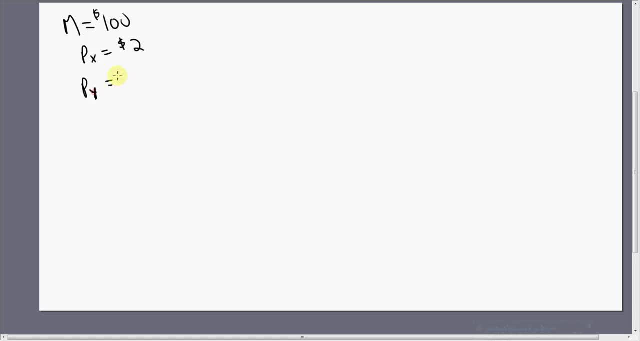 and the price of good Y equals $4.. This time, let's say, you have a $20 gift card for good Y. Okay, you're given a $20 gift card that can be used to purchase good Y. Okay, let's think how this may work.